Hello Linear Algebra, Good to see you again. How are you doing? Hopefully you are doing well. I am doing well also because today we'll be talking about symmetric matrix. This right here is actually not so bad, because the definition is just going to be: this is a square matrix. 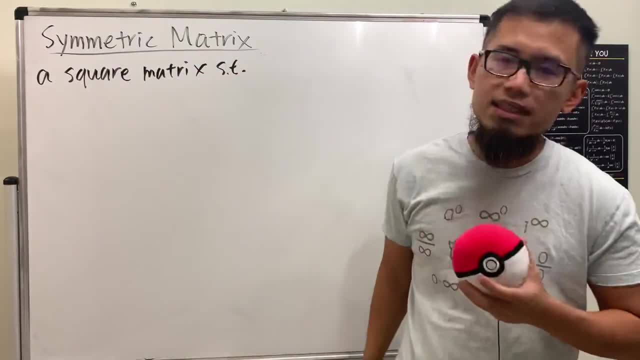 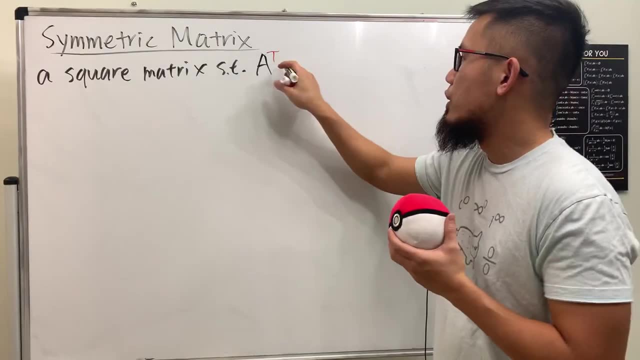 so that S dot, T dot, right. If you look at the square matrix A and then if you do the transpose to it, if the matrix is symmetric, you will just get a back Pretty cool, right, And you know what's. 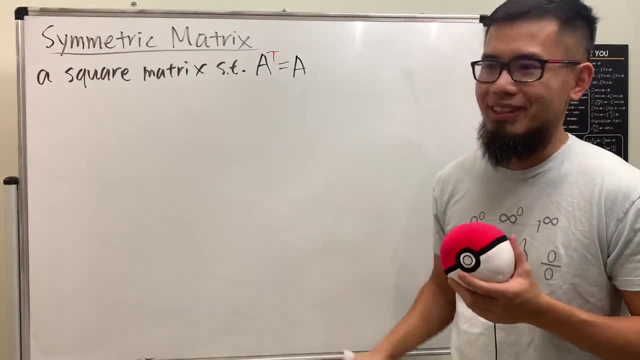 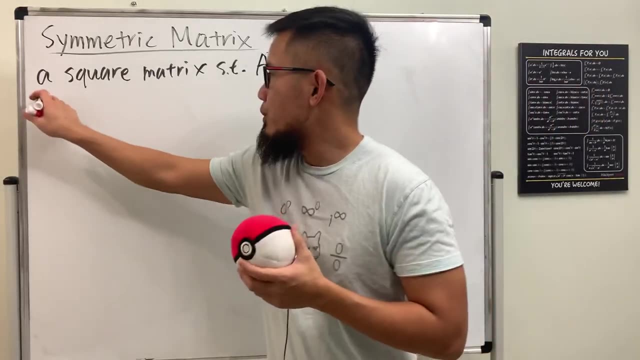 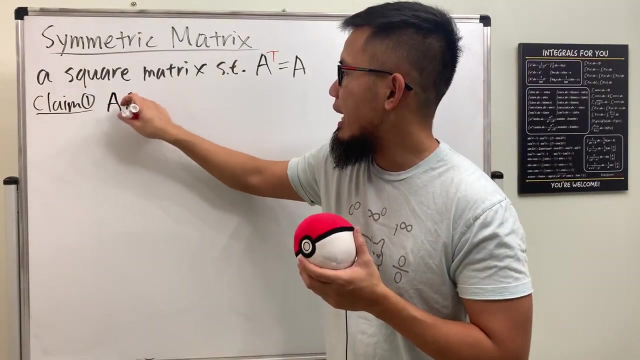 cooler than this, Some of the problems based on this right here, And I'm going to show you guys two of them and I will also ask you guys a question for you guys to think about. So I'm going to give you guys my first claim. Well, if you look at A times, A transpose, and in this case, 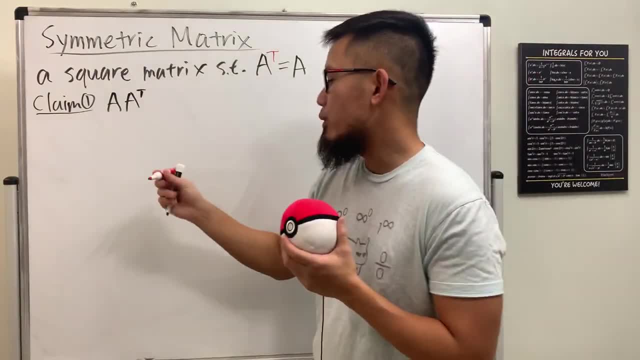 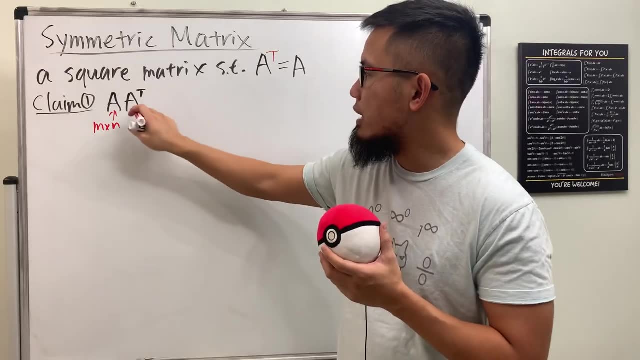 the dimension of A can be anything. So I'm going to write this down right here: A can be m by n, m by n, because if you do the transpose, this will become n by m, And when you multiply them, the result will be m by m. 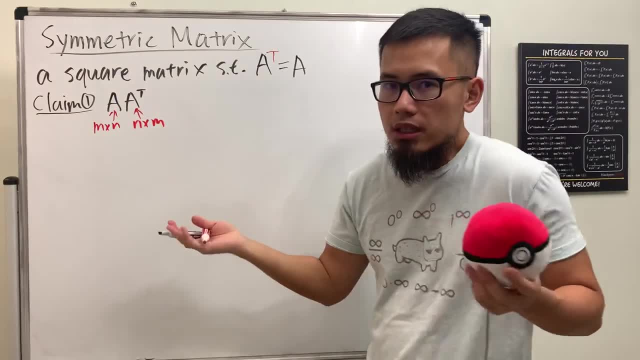 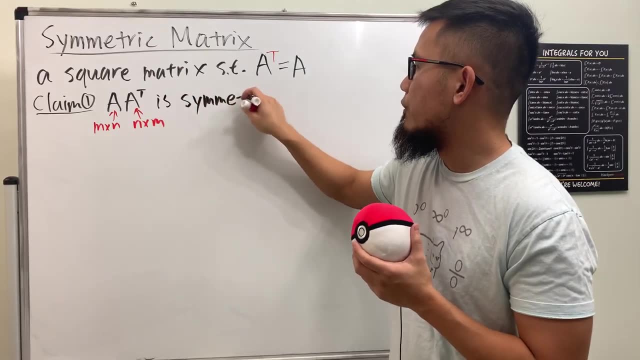 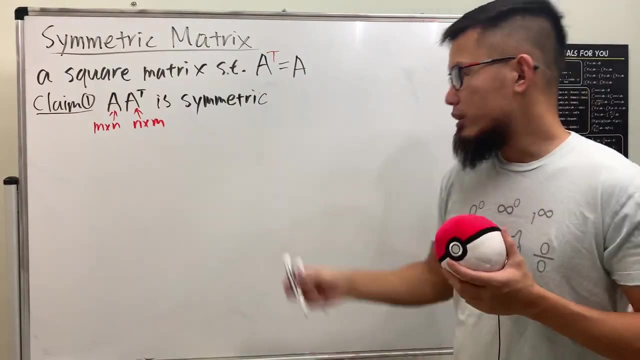 not m and m, m by m. So you know this right here And this it has a chance And in fact this right here is always going to be symmetric for any matrix A, not symmetrics Symmetric with a C at the end. So this right here is actually pretty cool. And before I show you, 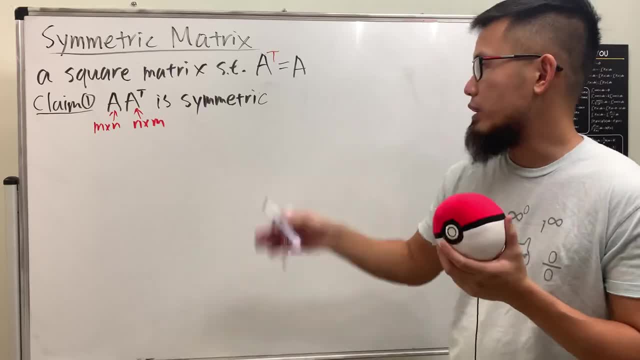 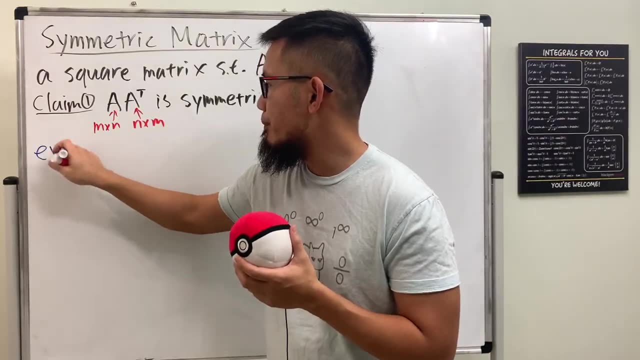 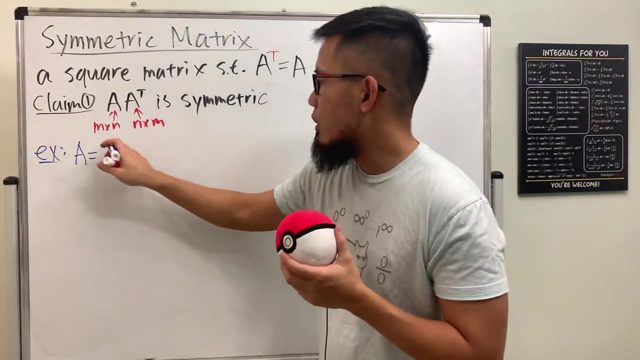 guys how we can prove this. let me give you guys an example, so that we can at least see how does a symmetric matrix look like. So right here, this is just a blue example. I don't know why it has to be blue, but anyway. Let's say A is equal to a 3 by 2 matrix. So I'm going to have the following: 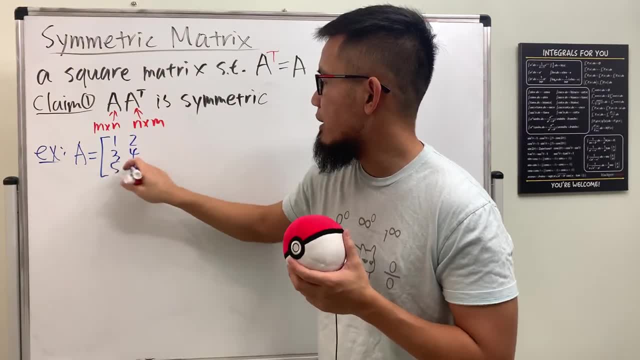 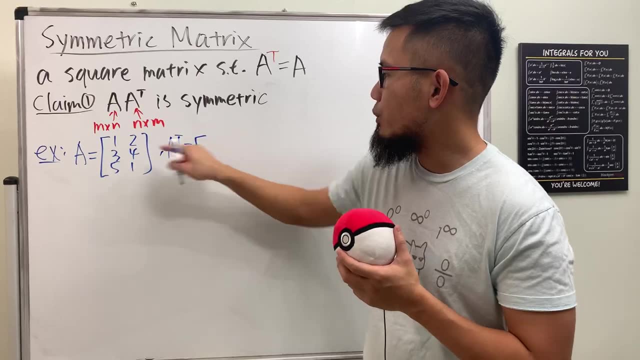 Let's say 1,, 2,, 3,, 4,, 5, 1.. All right, have a look, In this case A transpose. it will be just well, we do this and then put that as a column, So we 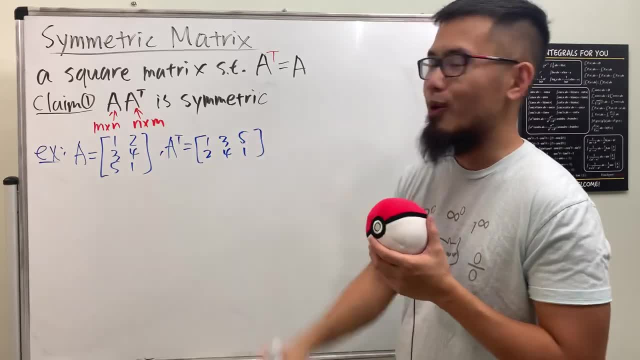 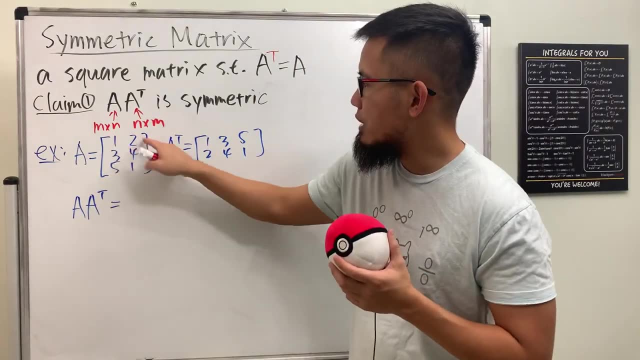 have 1,, 2,, 3,, 4,, 5,, 1, like so. And now, if we do A, A transpose, well, remember the order We have to do this times that. So here we go For the first entry, 1 times 1,, which is 1, and then plus: 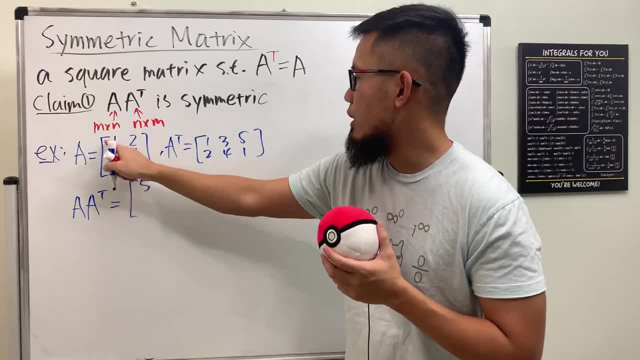 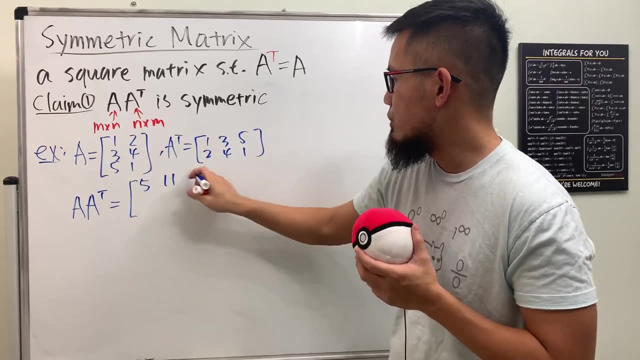 4,, which is 5.. So that's the first one, And then just continue, That's 3 and 8,, which is going to be 11.. And then 5 and 2,, which is 7.. And then this right here is going to be 3 and 8,, which is 11.. And 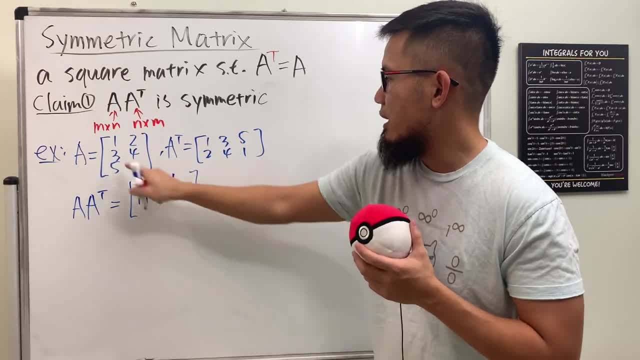 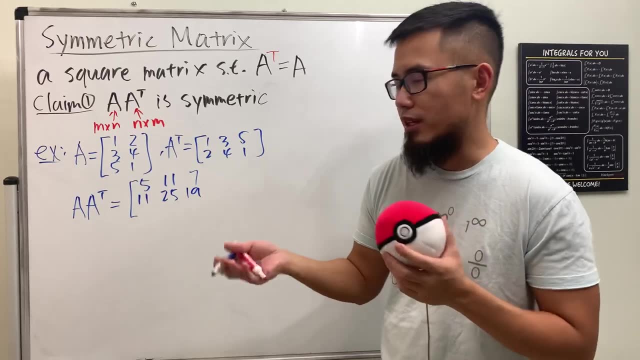 this is going to be 9 and 16,, which is 25.. And then 15 and 4 is 19.. And the last one: you can actually know the answer already, except for the last number. But let's see: 5 and 2 is 7.. And then 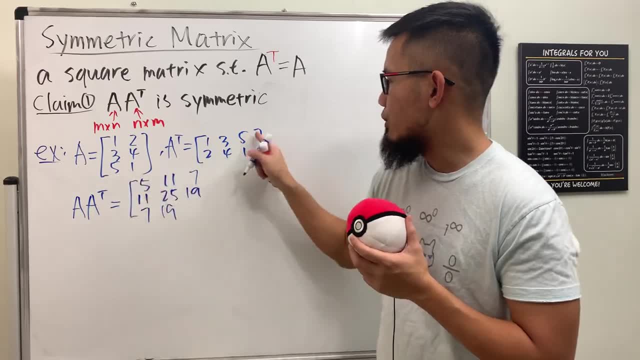 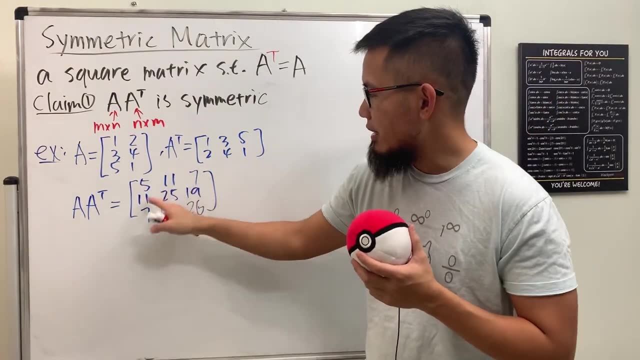 15. And that is 19. And then 25., And then 26., And then 27. And then 28. And then 29., And then 30. And 25. And 1 is 26.. Have a look right here. If you do the transpose this and that are equal. So it's. 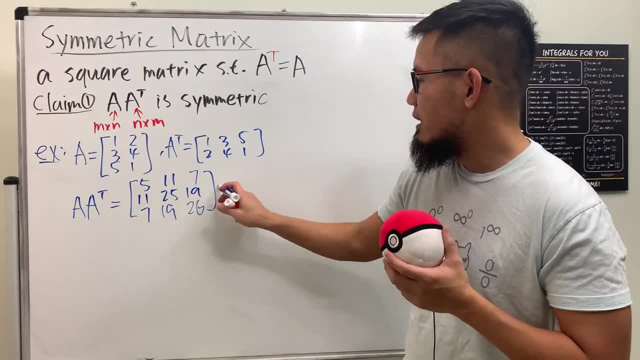 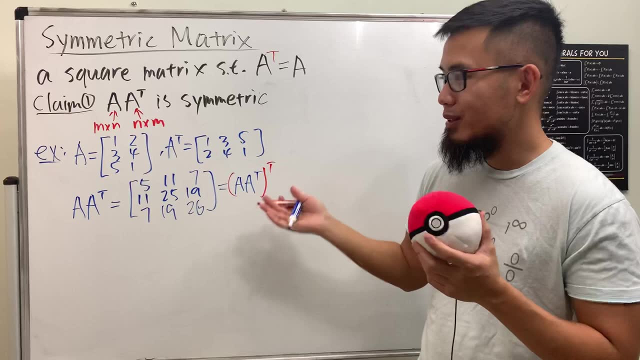 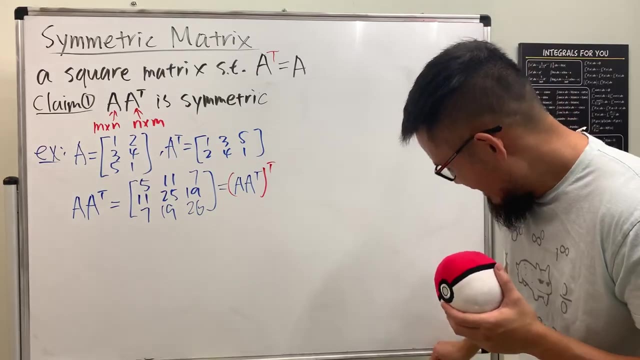 this and that, So it's this and that. So you will really see this will be equal to A, A transpose, and then you do the transpose Right. So hopefully this right here will convince you, But unfortunately an example is never the proof. That's the sad part, right? Otherwise it will be. 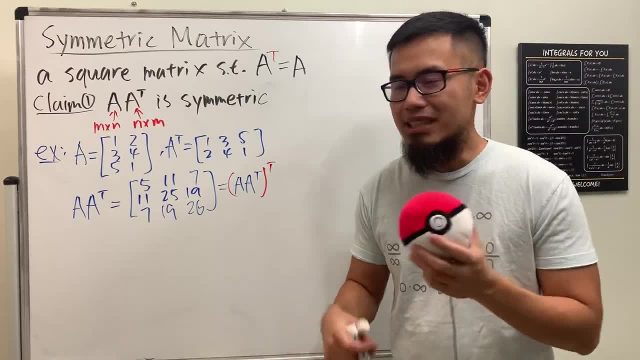 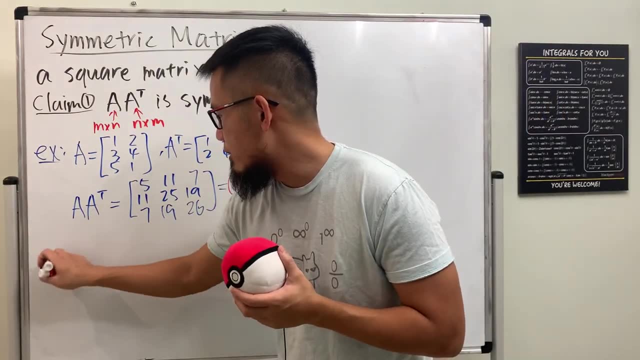 done already. Okay, The proof is actually not so bad. It's kind of based on the things I talked about in the previous video. If you haven't checked that out, go ahead and do so. So here is my little proof for the little claim right here. Well, you have to remember the definition whenever you're doing. 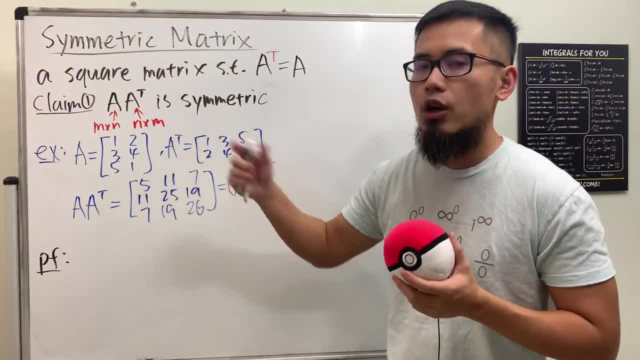 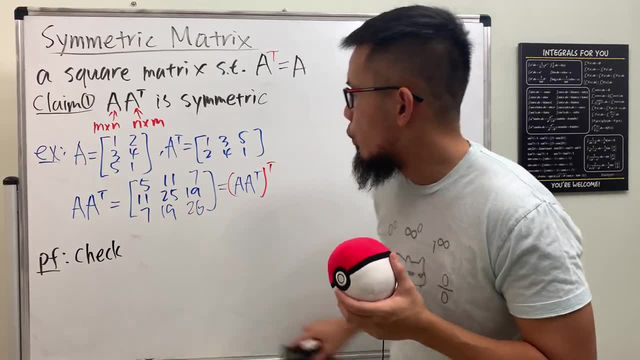 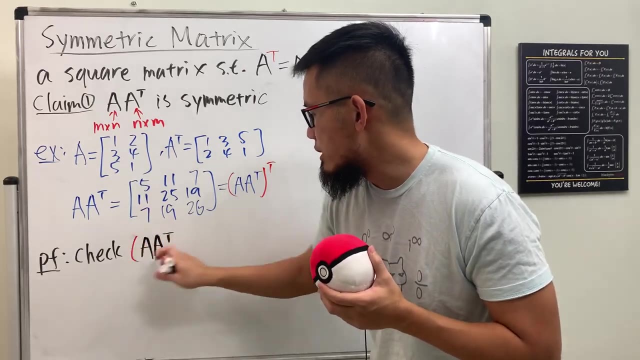 proofs. So if you want to say that this is symmetric, all we have to do is we have to go ahead and check what do we get if we put A- A transpose right, A- A transpose And then do the transpose to this guy. So this is what we have to check And hopefully by doing. 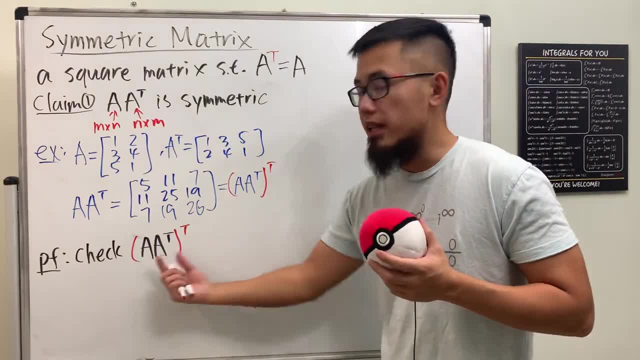 whatever we need to do, in the end we can just do that. We can just get it inside back. So that's the idea. You see, when we do A transpose, we just get it inside back. That's the idea, right. 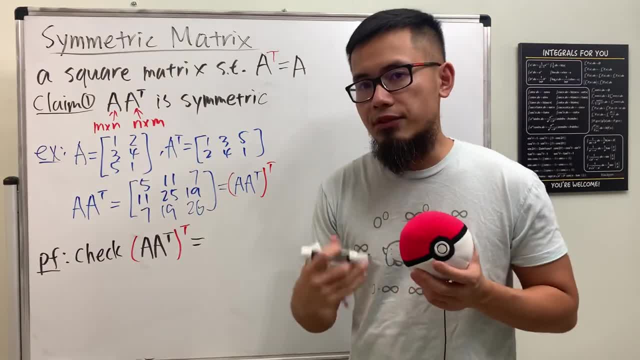 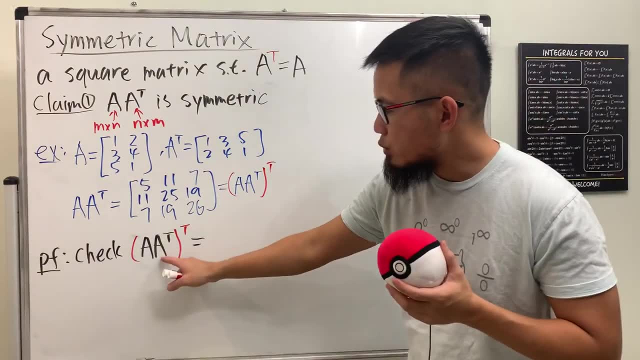 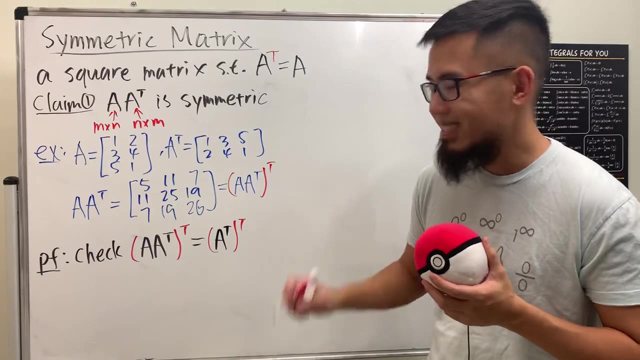 Now here is the deal From the last video. we talked about it. When we have a product of two matrix and then we do the transpose, what we get is this right here actually comes first. Now we get A transpose and then you do the transpose, all right, And then you put this right here. 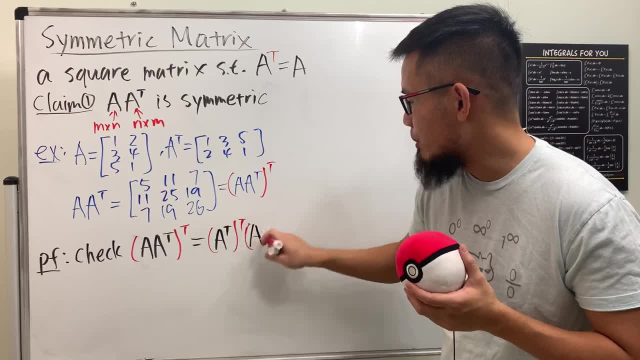 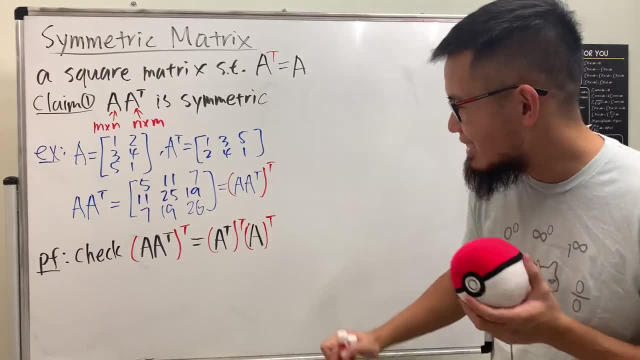 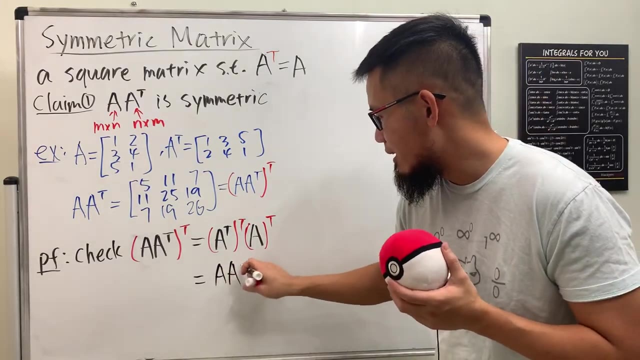 which is just going to be A, and then you do the transpose. All right, Now have a look: A transpose and transpose is just the A. right. So here, this is just going to be A, and then A transpose is just A transpose. Can you believe it? This is right. here, It's actually the proof. 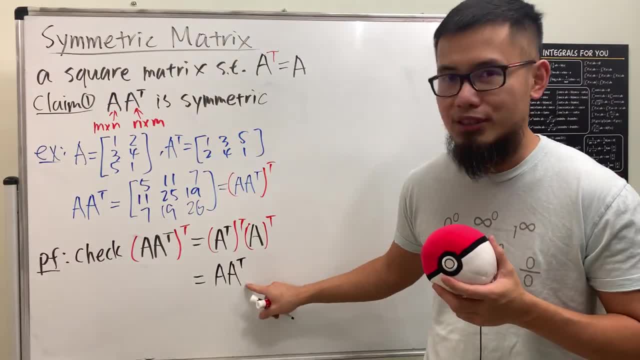 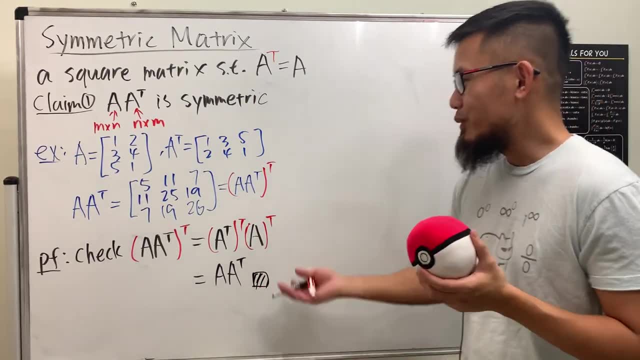 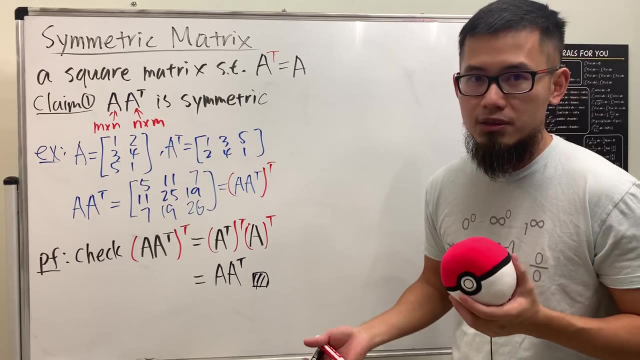 Have a look Inside. outside: Same Done, That's it. Very, very cool, huh, All right. So hopefully you guys can get this kind of questions on your test so that you can get the questions right. Pretty easy proof. But if you don't know the definition, you have no chance. 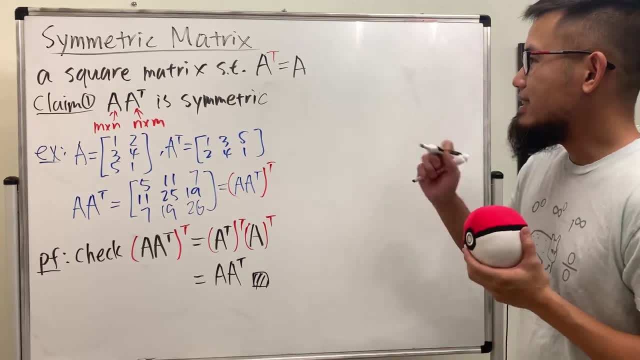 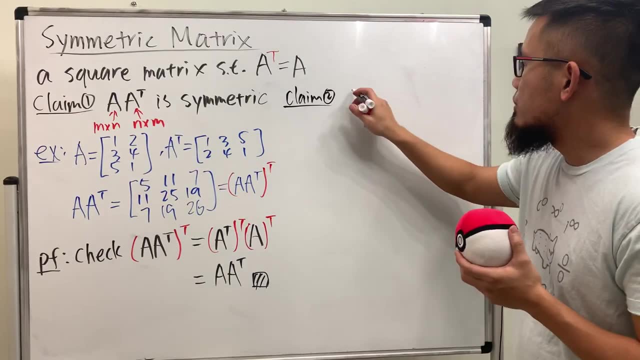 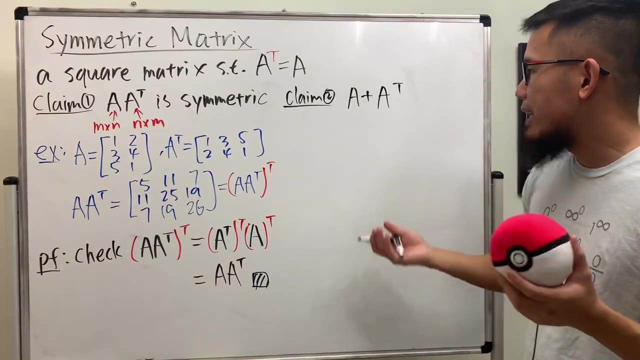 I'm very serious, right? So that's the first thing, And now let's look at claim number two. So for this one, let's look at A plus A transpose, And in this case, because we want to make sure that when we add the matrices, 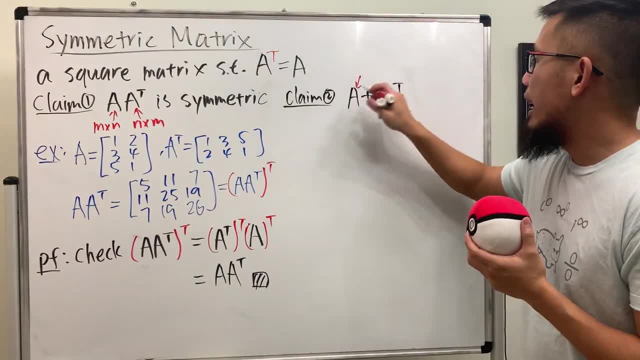 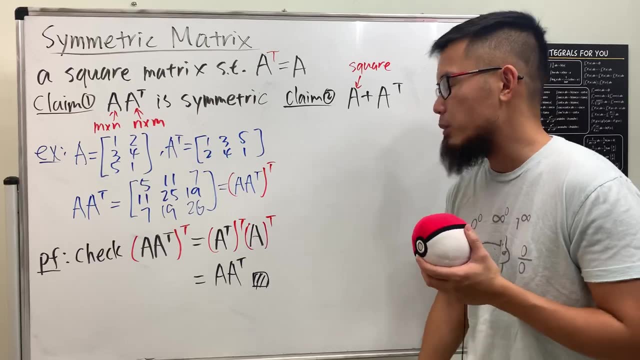 the dimensions have to be the same. So in this case, A and A transpose, of course A. in this case it has to be square, So you can say: that's an n by n or n by n, whichever, by whatever. They have to be the same thing in order to make this work. 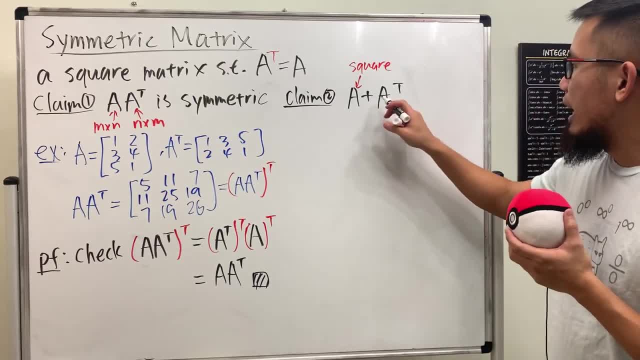 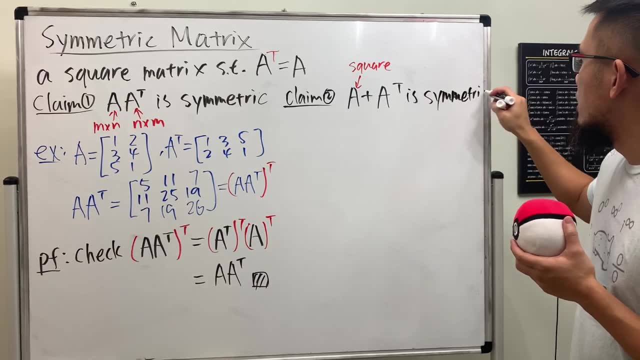 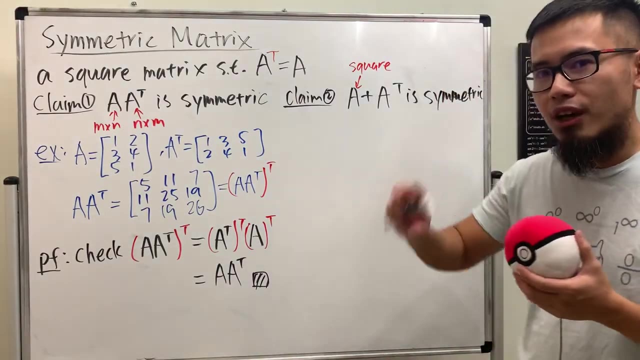 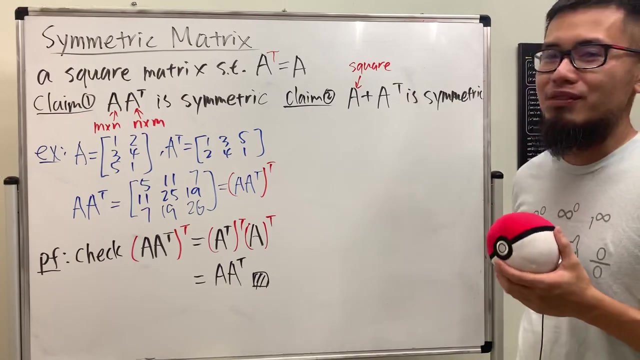 Believe it or not, if you add A and A, transpose this right here is also symmetric All the time. So if you have a matrix that's not symmetric, don't be upset. All you have to do is find, transpose and add it to the original. The result will produce a symmetric matrix for you. 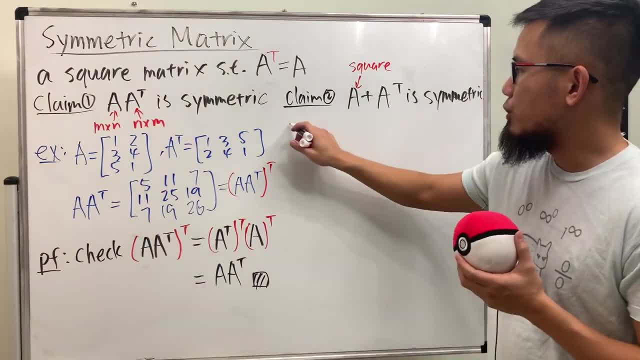 So for this one, I'm not going to do the example, I'm going to skip that. I'm just going to jump right into the proof, Very similar to what we have to do over there. So I'm just going to tell you. 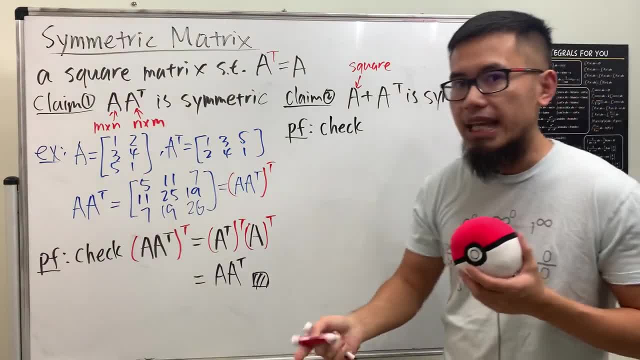 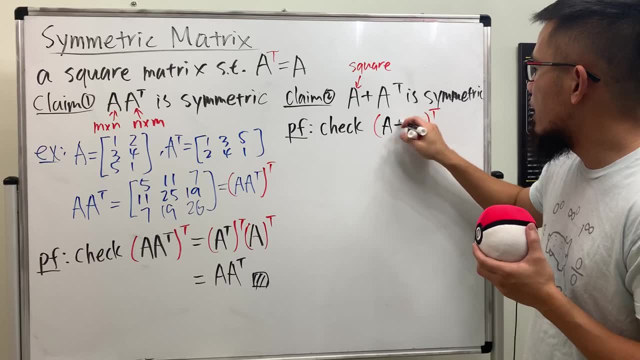 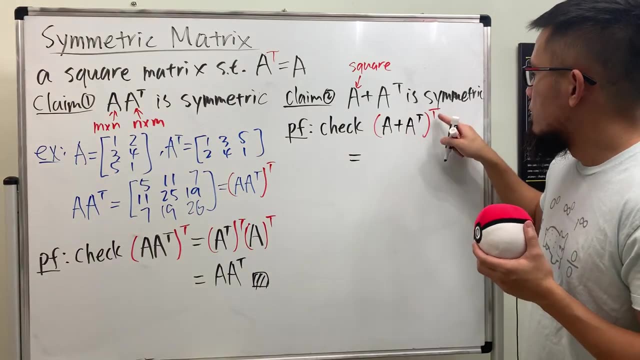 go ahead and check, Put this in and then do the transpose right. So put this, transpose that and then this right here inside. So a plus a transpose like: so: All right now, the sum, the transpose of the sum, is the sum of the transpose. 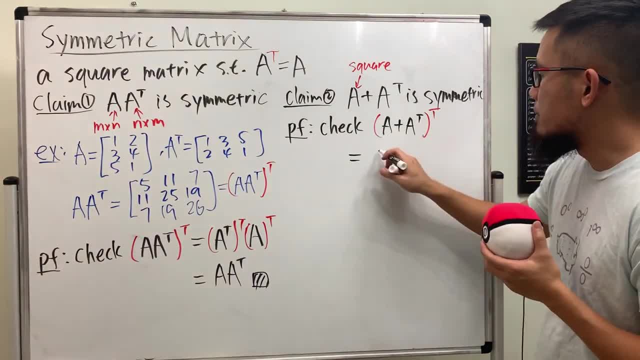 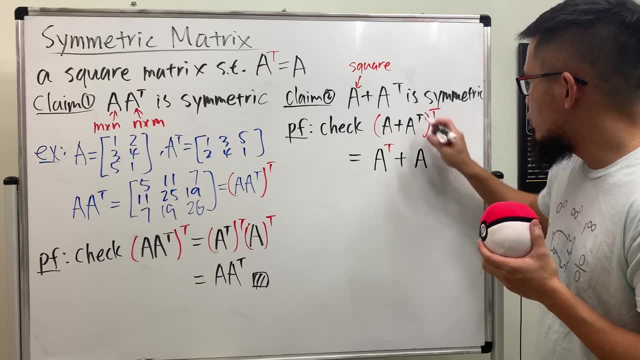 And again we talk about it last time. So this right here becomes a right. The first one, transpose that, and then we just have to add a transpose and then we transpose this guy right. So make sure you show each and every step. 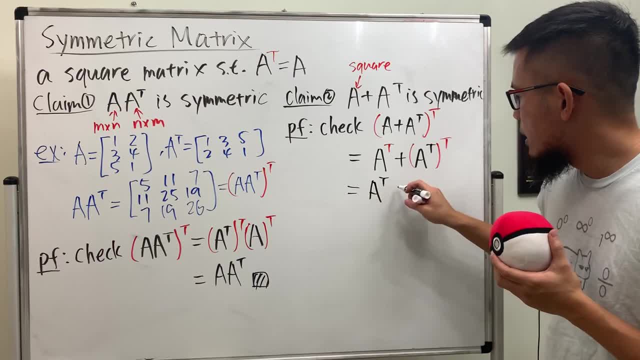 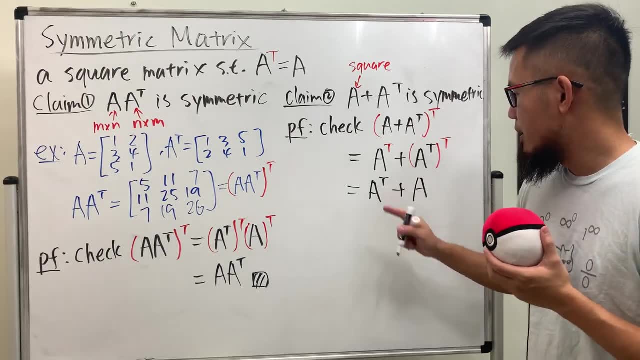 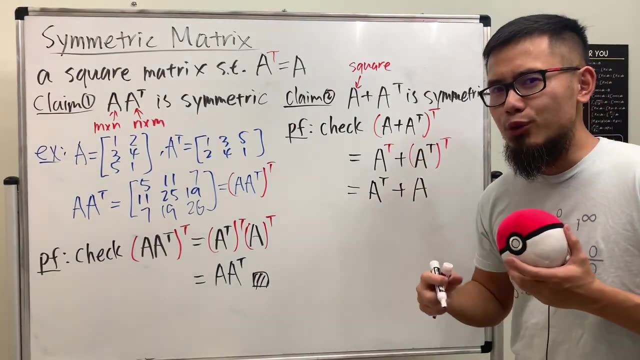 All right, this guy is just this guy. so a transpose, but a transpose, transpose. this is just the a by itself. And have a look, a transpose plus a is not the same as the original inside. Yes, but if you want to write down a nice proof, 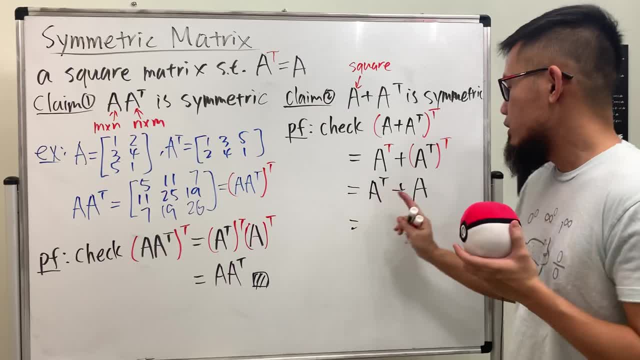 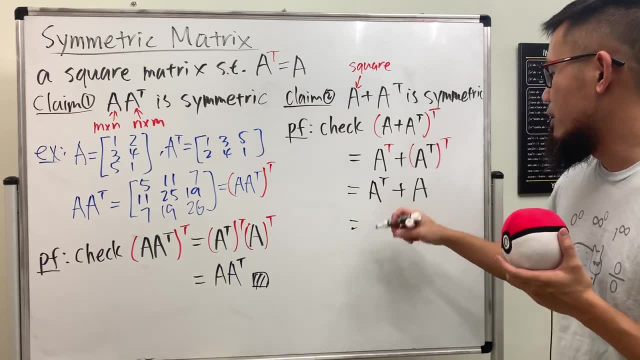 what you have to do is switch the order, and we can, of course, switch the order of the first and the second Of the sum of matrices- that's totally okay- But we cannot switch the order of the product of a matrix. 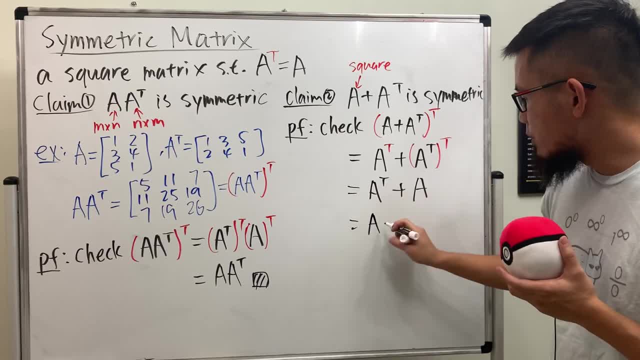 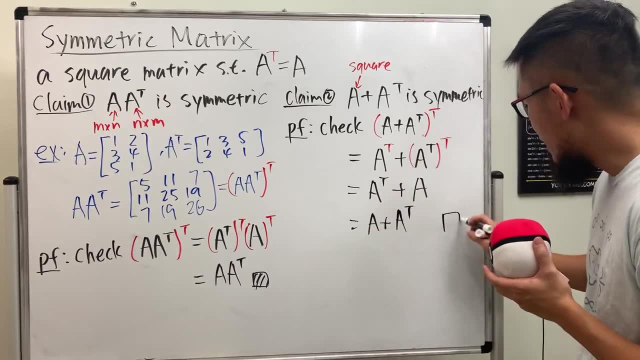 So in the end here we can just write down this: a goes first, and then this: a transpose goes next, and inside, outside done, And then again put a box just like that, Very, very cool, All right. so now you're going to kind of. 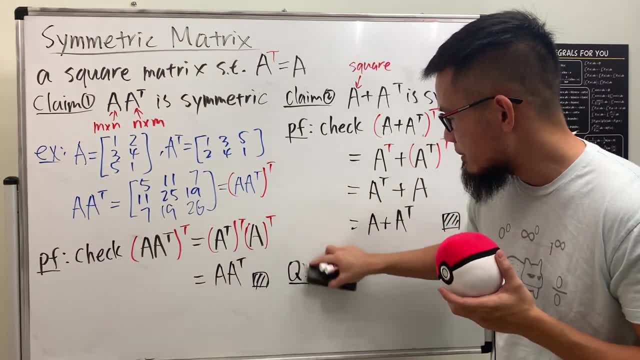 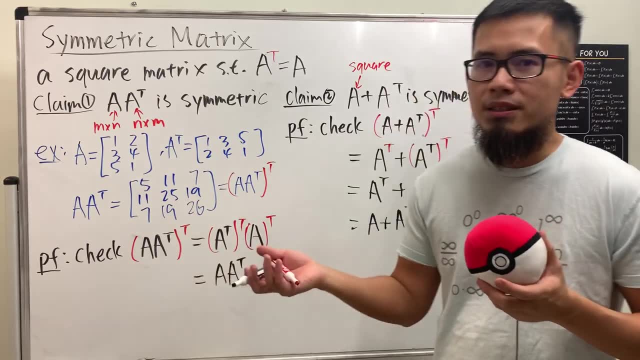 encounter this kind of questions a lot. So this is going to be a question for you guys, for you guys to think about. Think about: right whenever you have like a special matrix. right whenever you have like a special matrix, in this case, when you have a symmetric matrix. 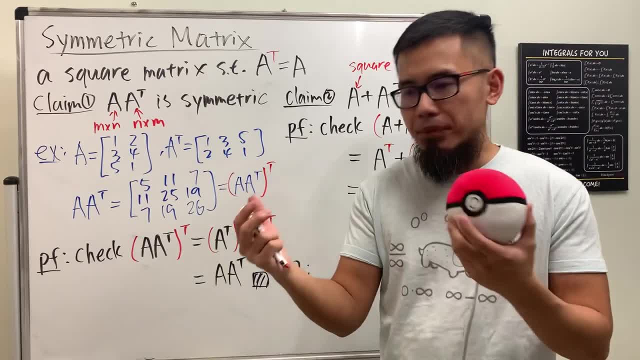 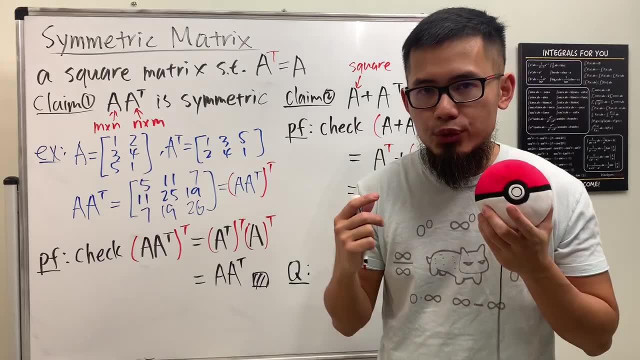 what people would like to do is that they will ask you if a and b, they are both like that special matrix, In this case the symmetric one. If you multiply them, do you get a symmetric matrix as well? So the question right here for you guys, right? 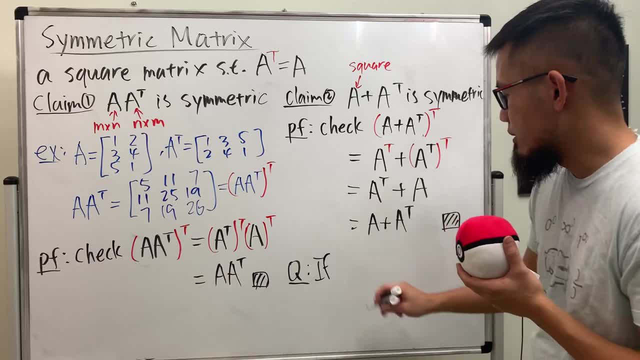 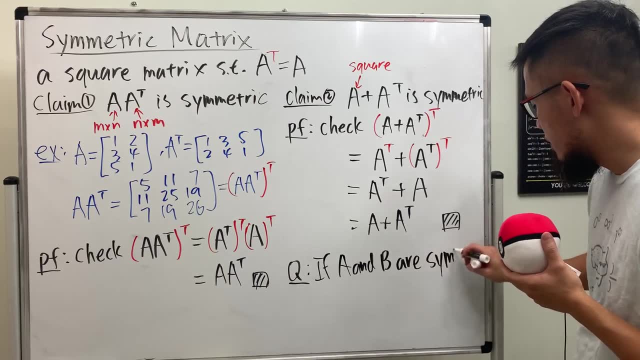 So if man there will be a lot of words, right. So if man there will be a lot of words, right. So if a and b are symmetric, Man, I just cannot write: Yeah, there we go. 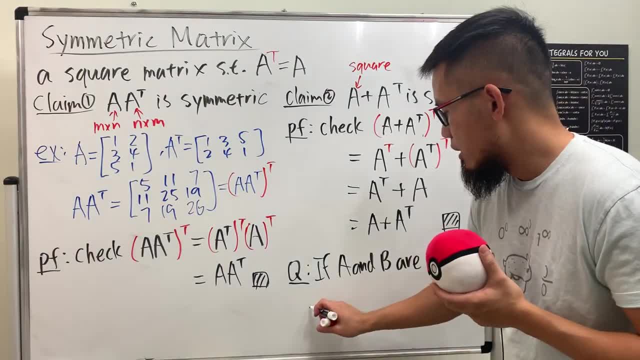 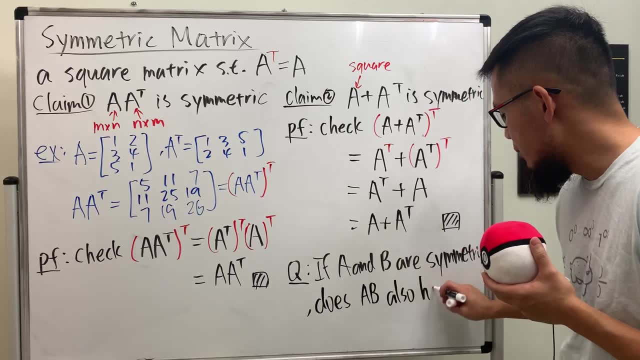 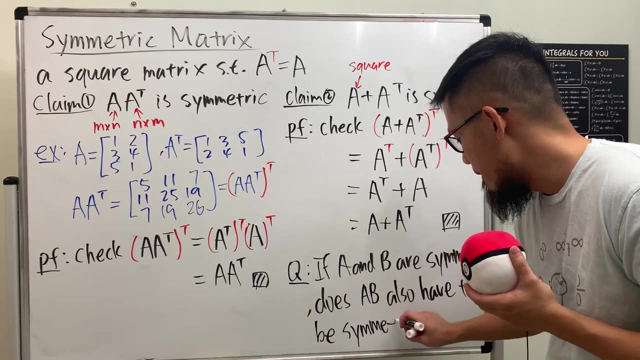